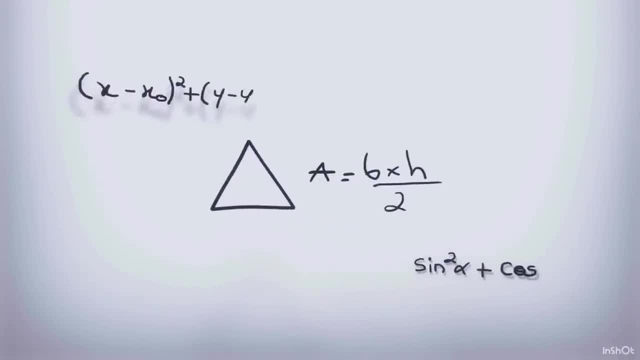 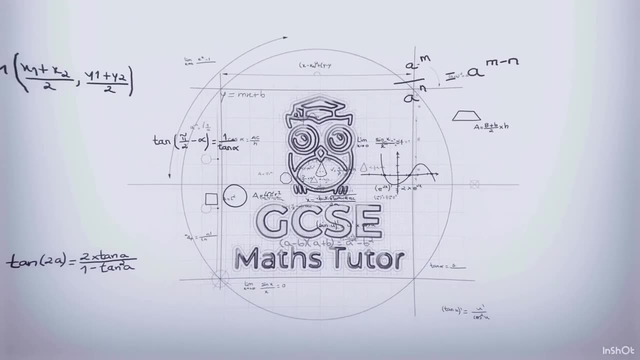 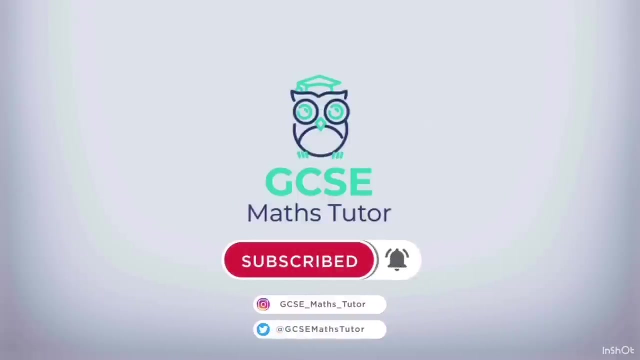 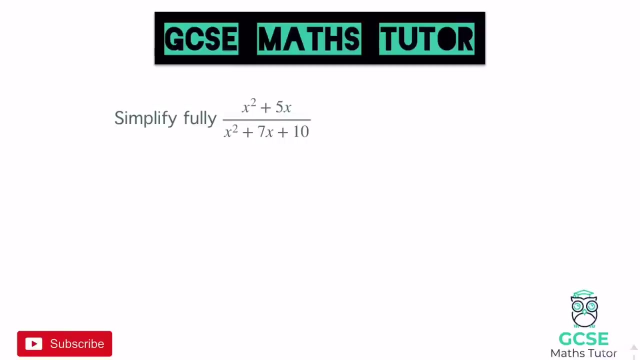 Okay. so in today's video we're going to have a look at algebraic fractions. Now we're going to have a look at lots of elements of algebraic fractions. We're going to have a look at simplifying, adding and subtracting and some dividing at the end. So grab a piece of paper, grab a pen. 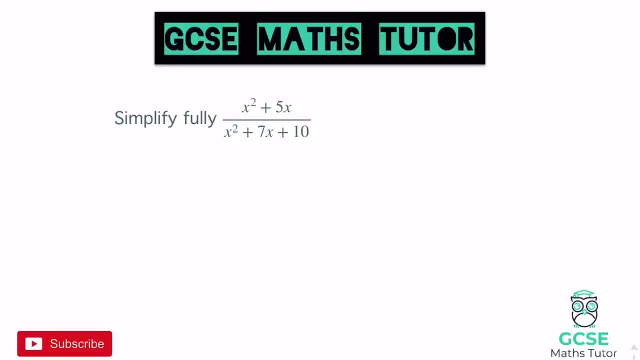 make some notes and we're going to get started on this question. So when we're simplifying an algebraic fraction, we're looking for a common factor on the top and the bottom When it comes to algebra, to find a factor. in algebra, we can factorise to find a factor. So if we have a look 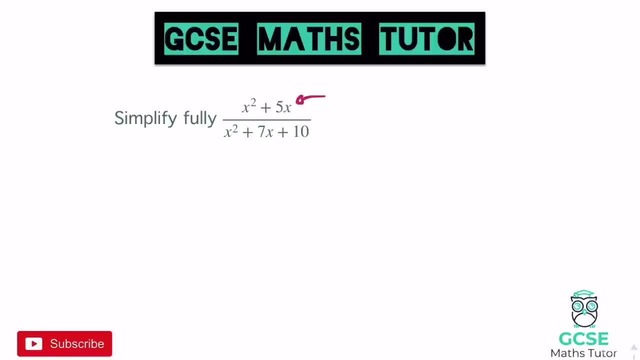 at the top and we just need to factorise both of these. now the expression on the top there has an x in both, So we can factorise this by x. No numbers in both, but we can factorise it by x. 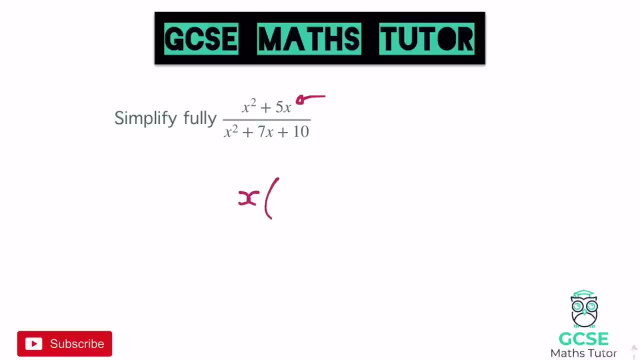 So if we take x out of the bracket, we would have x, and then inside the bracket we'll have x minus- sorry- plus 5.. Okay, x plus 5.. If we do the same on the bottom, we've got a quadratic on. 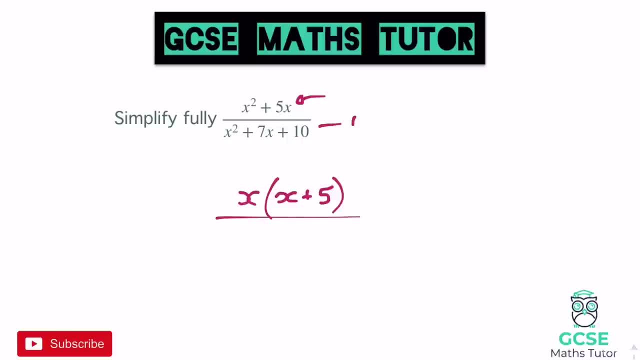 the bottom. so you need to know how to factorise quadratics here. But we've got 1 and 10, or 2 and 5 as our options to go in our double bracket And in order to make 7 there in the middle. 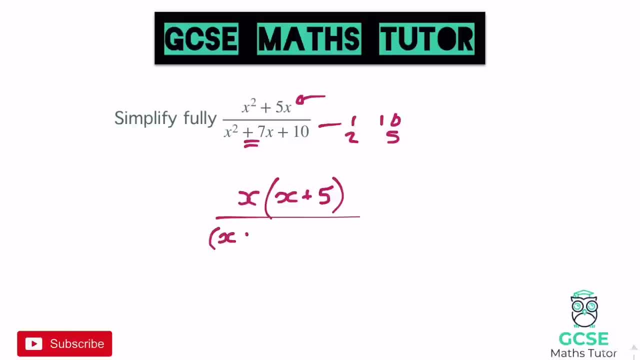 we want plus 2 and plus 5.. And here we go: x plus 2 and x plus 5.. There is a little bit of a hint in terms of the factors we'd be using, because obviously we had x plus 5 on the top, but it's not. 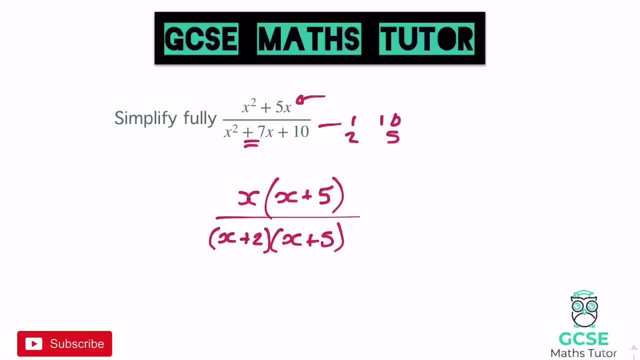 always going to be the case that we'll get that, But obviously so we still need to be able to factorise. but there is a little bit of a hint there that there was going to be an x plus 5 in one of the brackets. Now there's an x plus 5 on the top and the bottom, so essentially what we can. 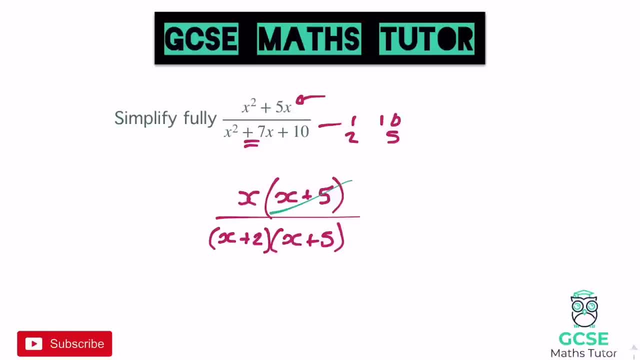 do is we can divide the top and the bottom by x plus 5, which would cancel out these brackets here. And if we cancel them out, we just need to write what's left. We have x on the top, and on the bottom we have the x plus 2, which you can either put in the brackets or leave without the brackets. 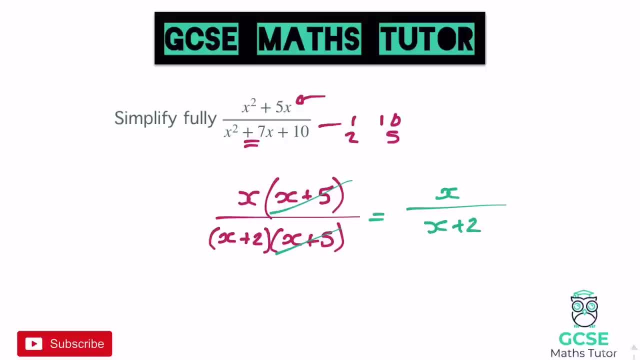 it doesn't matter there, But our final answer is x over x plus 2.. Right, let's have a look at another one. Okay, so we've got another algebraic fraction here that has already been factorised on the bottom, So actually, let's have a think about how we'd approach this. Now we want to cancel off a common 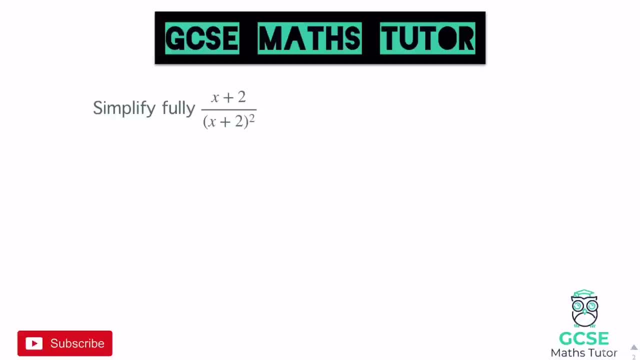 bracket or a common factor, and the top and the bottom both divide by x plus 2.. So actually, if we imagine what this would look like if we were to sort of expand that bracket or just write it as a double bracket, we'd have x plus 2 on the top, on the bottom it's x plus 2 and x plus 2 as a. 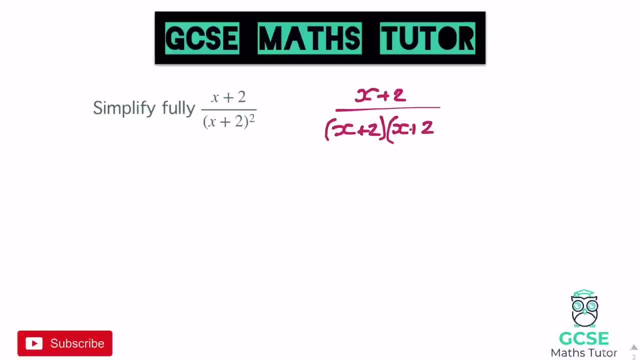 double bracket. There we go Right. so if we cancel off one of the x plus 2's top and bottom, we've just got to be careful this time so we can cancel that one off and it'll disappear. but not to forget, we are dividing by x plus 2.. 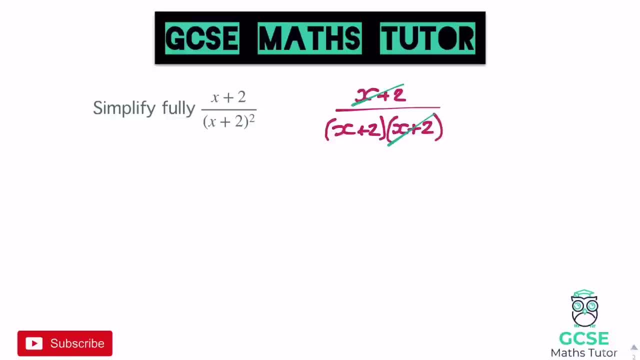 So when we cancel the one off the top, it doesn't just disappear, but if we divide it by x plus 2, it becomes 1.. So, writing our final answer, we would have one on the top and x plus 2 on the. 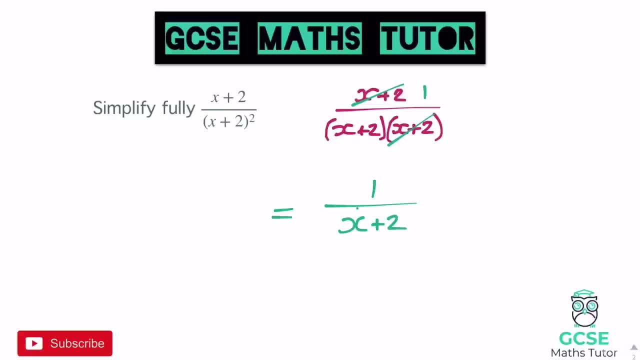 bottom, which again I'll just get rid of the bracket there. so 1 over x plus 2.. So just watch out with these sorts of questions here. when the factor is all that there is on the top, Obviously that does become a 1 there, it doesn't just disappear. 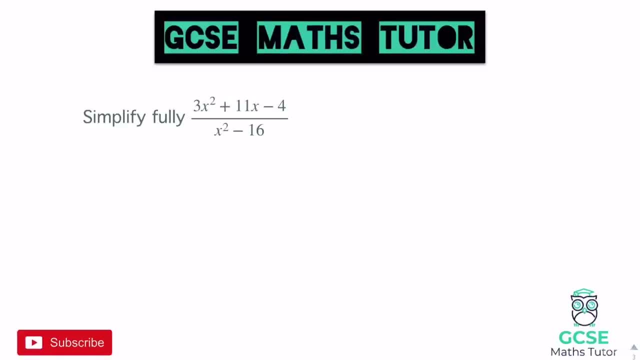 Let's have a look at one more before we have a go. OK, so in this question we've got a slightly harder quadratic on the top and a different sort of quadratic on the bottom. So on the bottom there, hopefully you recognise that it's a difference of two squares. 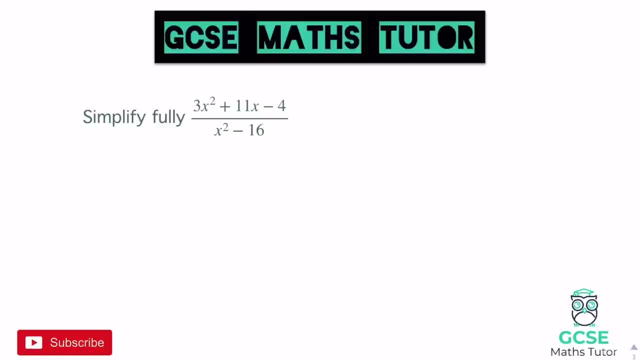 When there's no x piece in the middle. there it's because the numbers are the same and they've cancelled each other out. So if I start with the bottom, I just think it's the easier one there. the factors of 16 that are the same are 4 and 4.. 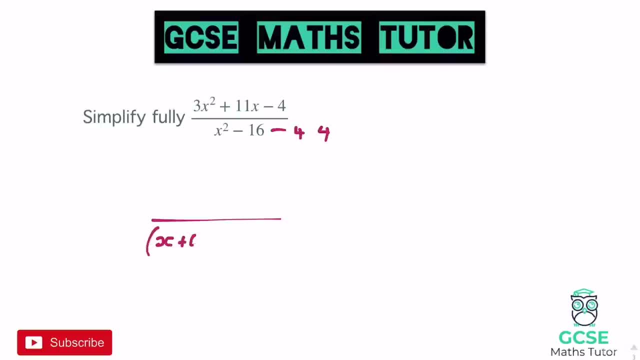 So our difference of two squares there is x plus 4 and x minus 4.. There we go, and that's that factorised on the bottom. That gives us a little helpful hint for the one on the top there which is slightly harder. 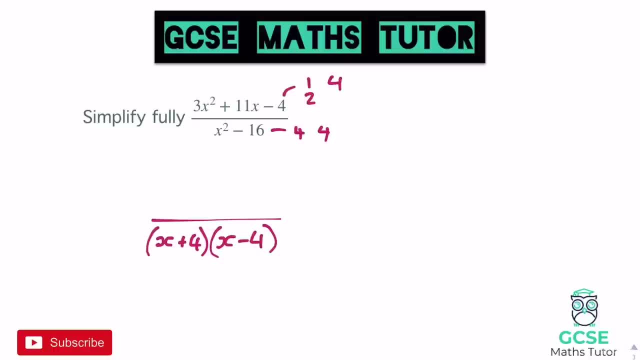 because our factors of 4 are 1 and 4, or 2 and 2. And because we've got the little hint here that we know we're going to have a 4. if it's going to simplify, we know it's going to be the 1 and the 4,. 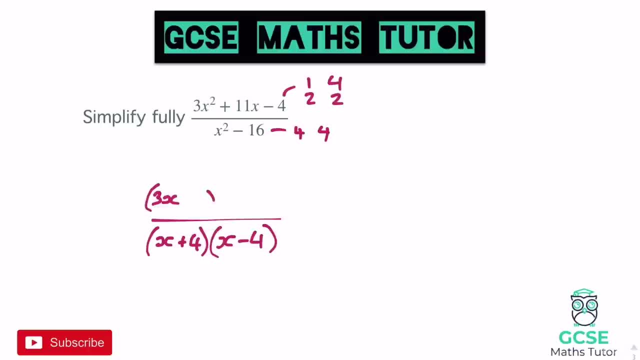 but then we just need to have a look and figure out which way it goes round. So we've got 3x in one bracket and an x in another. That'll allow us to get the 3x squared Again, obviously. check out my video on this. 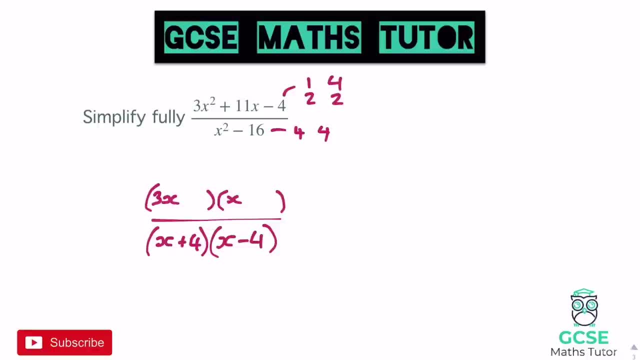 I'll be on factorising these quadratics or harder quadratics, if you're unsure on these. But in order to make 11 there, we're going to want the 4 to get multiplied by 3 to make 12.. So we want plus 4.. That'll make positive 12.. 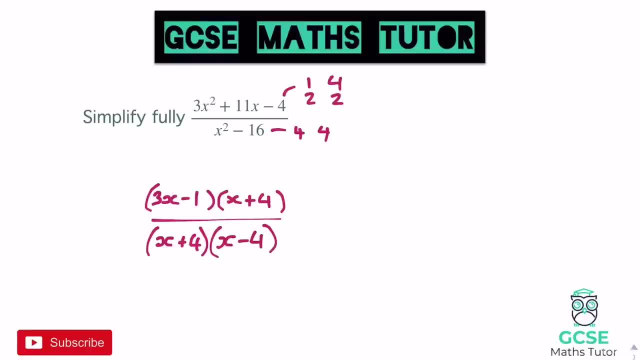 And we want to take away 1, so we'll put the minus 1 over here in the other bracket And again, now we've got it factorised, it's nice and easy for us to cancel off these x plus 4s. 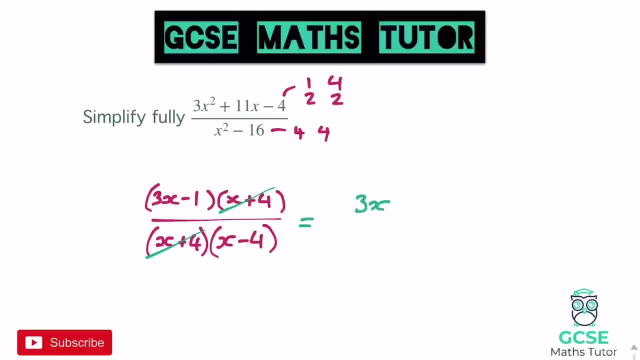 and just write what we've got left. On the top we've got 3x minus 1.. And on the bottom we've got x minus 4.. And there we go. That is our fraction there, Simplified Right. here's some for you to have a go at. 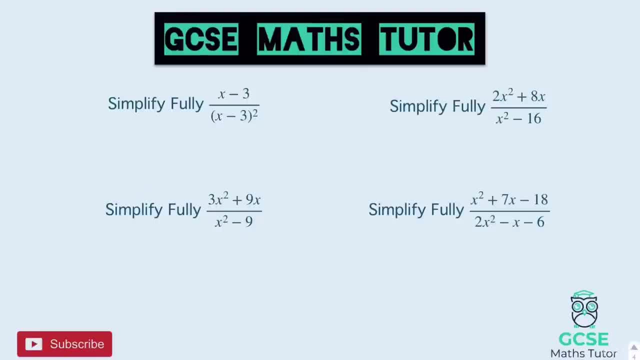 OK, so four questions. Have a go at these. pause the video there and we'll go over the answers in a sec. OK, so for the first one we can cancel off an x minus 3 on the top and the bottom. 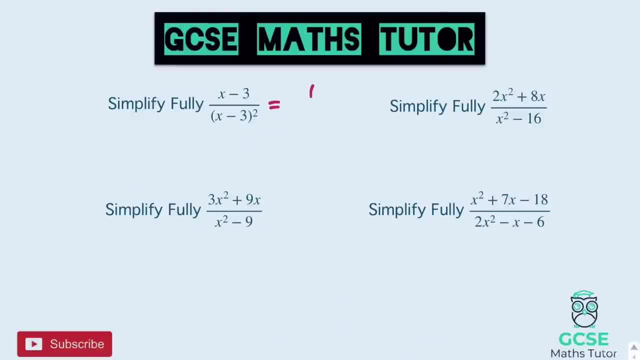 So if we cancel off an x minus 3 on the top, we're left with 1. And if we cancel one off the bottom, we've just got one of them left. So we've got x minus 3 left on the bottom. 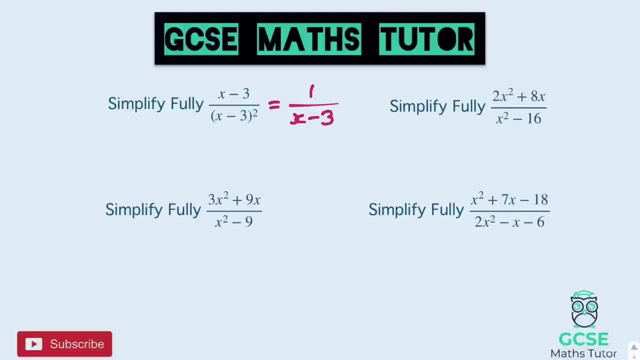 And that's our first question. Onto the second one: If we factorise these to start with now, that top one there factorises by 3x, So we've got 3x out And on the inside then we would have x minus- sorry- plus 3.. 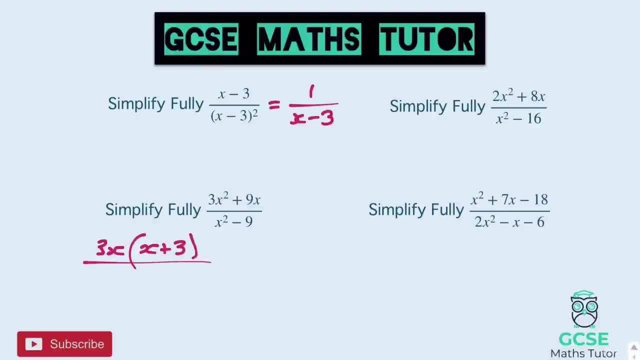 There we go, And on the bottom we've got a quadratic. It's a difference of two squares, So it's x plus 3 and x minus 3.. There we go: x minus 3, x plus 3.. And then again we can cancel off top and bottom. 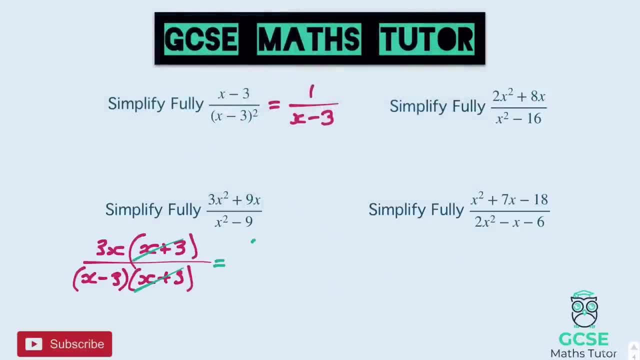 So if we cancel off these x plus 3s, what we're left with is 3x over x minus 3. And there's our fraction. simplified Onto this top right, We've got 2x that we can bring out the brackets. 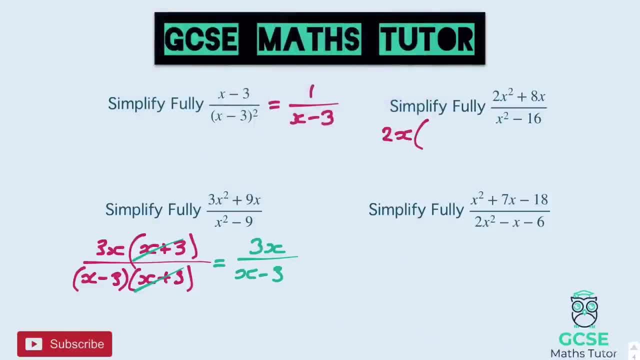 So if we factorise that by 2x, we'll get x plus 4 on the inside And on the bottom. there again we've got a difference of two squares, So it's x plus 4 and x minus 4.. 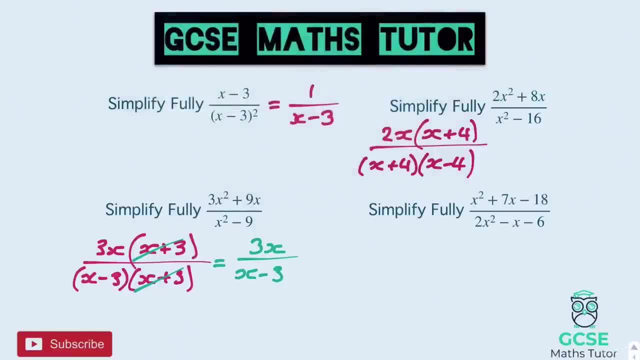 There we go, And those x plus 4s are going to cancel each other out And we are left with 2x over x minus 4.. There we go, And that's that one factorised and simplified. And onto the last one here. 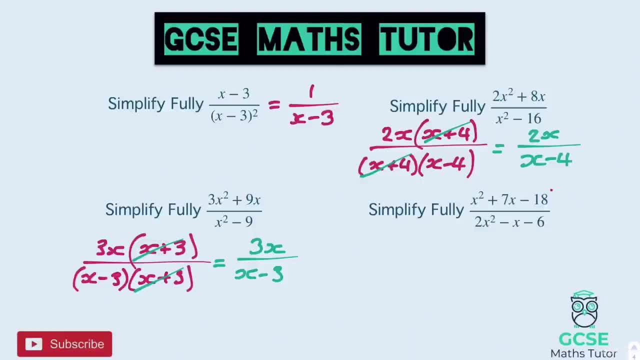 We've got two quadratics, So the factors that times to make 18.. We've got 2 and 9,, 3 and 6, or 1 and 18.. It's going to be the 2 and the 9, though, to make 7.. 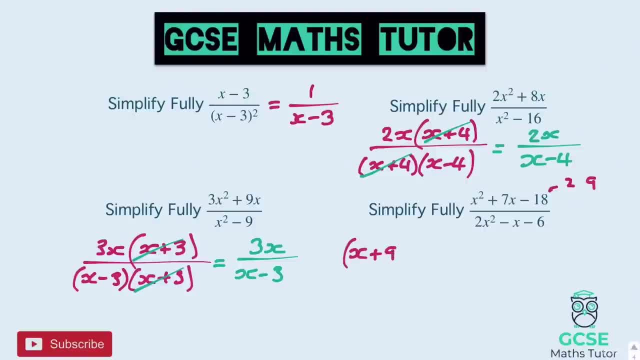 So we've got x plus 9. And then take away 2 to make 7.. So x minus 2.. And on the bottom factors that times to make 6. We've got 1 and 6 or 2 and 3.. 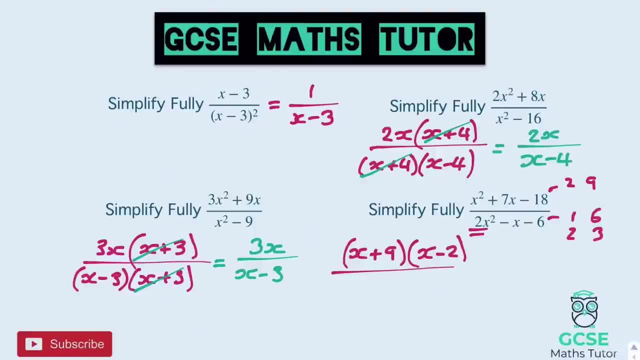 One of them is going to double because we've got the 2x squared there. So we've got 2x in a bracket And x in our other bracket And we're trying to make minus 1 in the middle. So in order to make minus 1, we can have 4 and 3.. 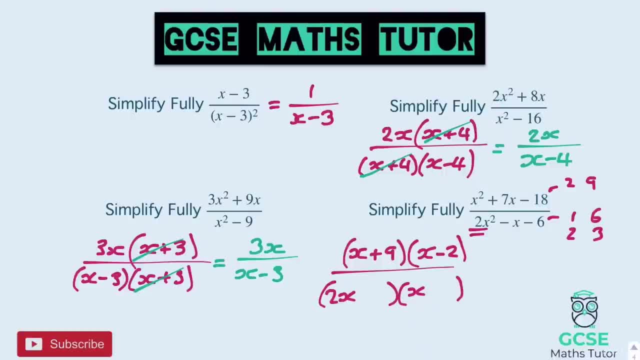 That works. if we double the 2. That would make 4 and the 3.. So we want positive 3.. Take away 4.. So let's have x minus 4 and x plus 3.. Sorry, that shouldn't be a 4.. 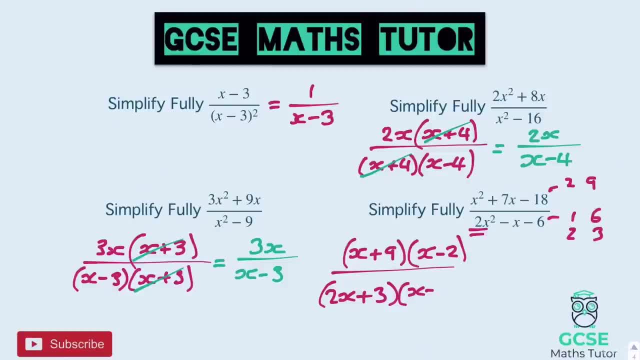 That should be a 2.. We're doubling it to make the 4.. So x minus 2.. There we go, And 2x plus 3. Just double check that. So 2x times minus 2 makes minus 4x. 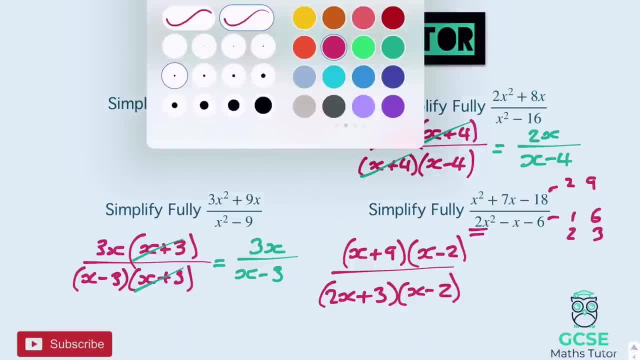 Add the 3x in the middle, That makes minus 1.. Right, there we go. Make sure you put the right numbers in there. I almost put the 4 in, So we are putting the 2 in there And then canceling off these x minus 2s. 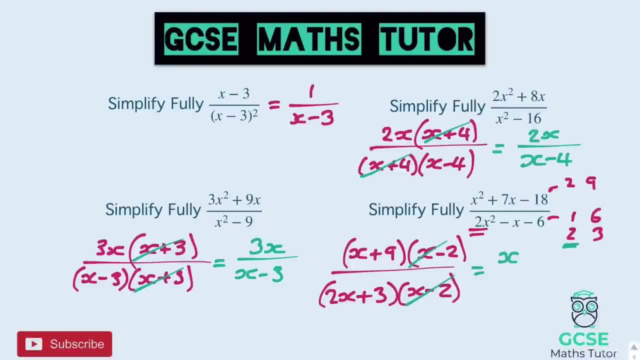 And that leaves us with x plus 9 on the top, And on the bottom it leaves us with 2x plus 3.. There we go, And that's simplifying an algebraic fraction. Right, we're going to have a look at some adding and subtracting. 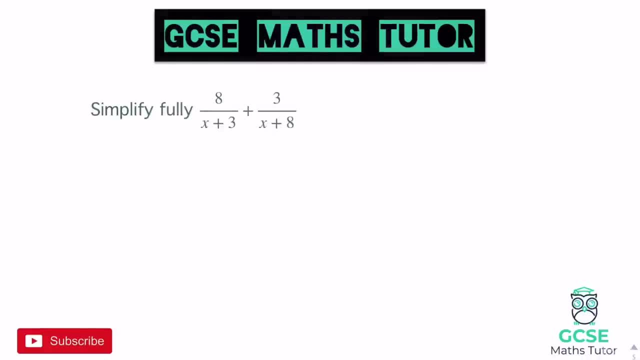 OK. so this says: simplify this fully. So we've got 8 over x plus 3. Add 3 over x plus 8.. Now what we need is a common denominator when we're adding fractions, just like we're adding normal fractions. 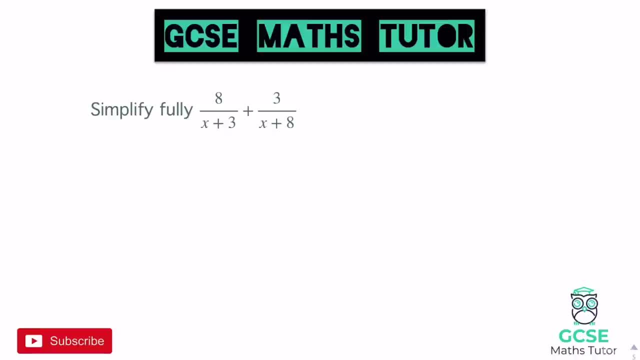 So I'm going to multiply the right fraction by the left denominator. So I'm going to times the top and the bottom by x plus 3, which I'm going to write in a bracket there. It's going to help when I actually multiply it. 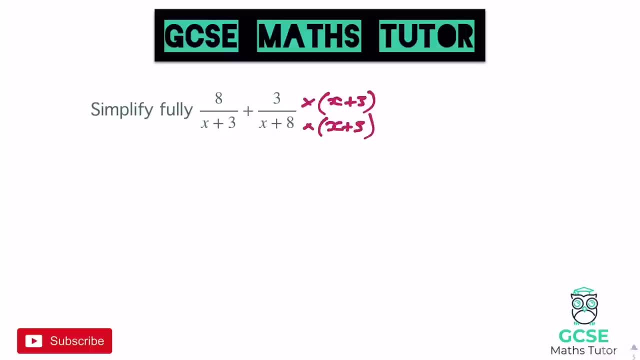 So times the top and the bottom by x plus 3.. And then I'm also going to times the left by the right denominator. So I'm going to times the left by x plus 8.. And also on the top, timesing that by x plus 8.. 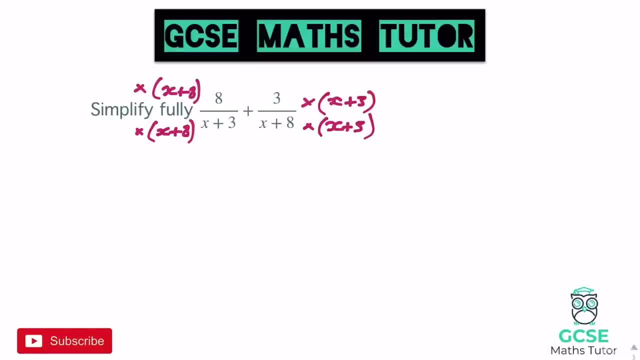 Just like with normal fractions here. So if we times the top there by x plus 8, we actually get a single bracket. We get 8, lots of x plus 8.. There we go Over and we've got a double bracket on the bottom. 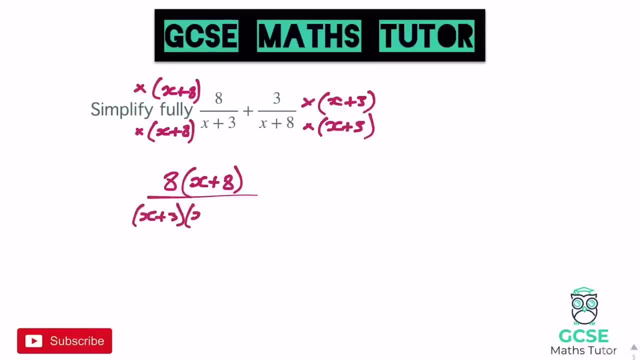 We've got x plus 3. that's also getting multiplied by x plus 8. And we are adding to that 3, lots of x plus 3.. And on the bottom we've got that double bracket: x plus 3, x plus 8.. 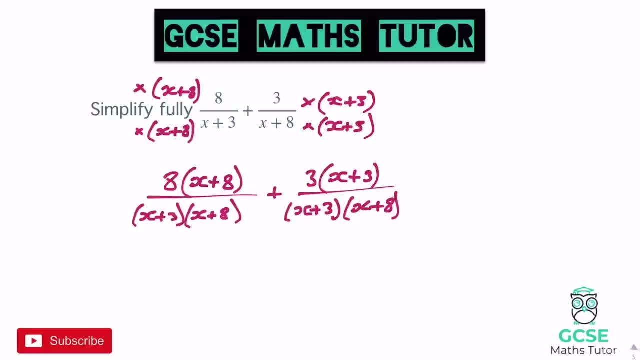 There we go: x plus 3,, x plus 8.. Right, so if we go back actually expanding these numerators and we can join it all together, So 8 times x and 8 times 8. And that gives us 8x plus 64.. 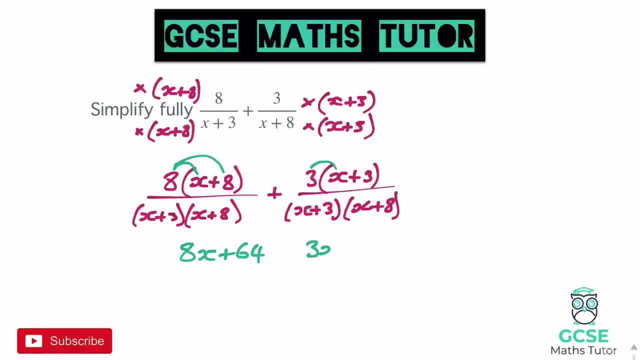 And on our other one we've got 3 times x, which is 3x, And 3 times 3,, which is 9.. There we go, And we're going to add these fractions together, So let's rewrite these denominators in. 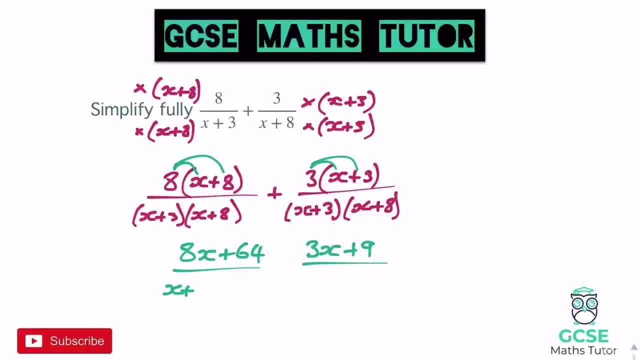 We've got x plus 3, x plus 8.. And another one: x plus 3, x plus 8.. There we go, And we're adding these together, Right? so if we add them together, we've got the 8x, add the 3x, which makes 11x. 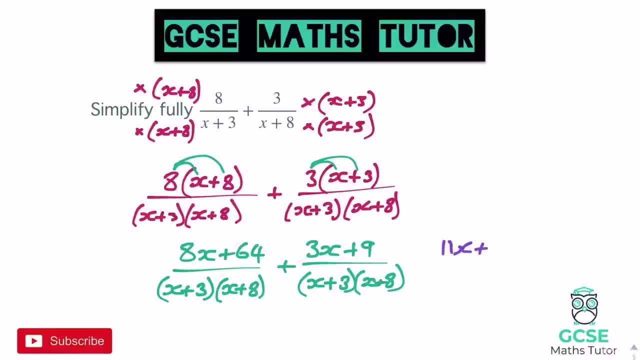 And we've got the 64. add the 9, which makes 53.. So 11x plus 53.. All over that denominator which we can expand or we can leave it in brackets if you do want to expand it: x times x is x squared. 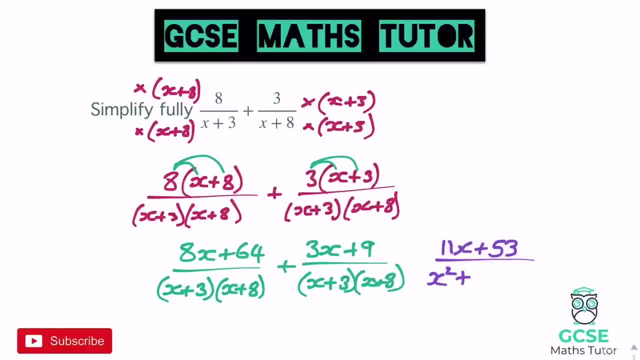 Times 8x and 3x. So we've got 11x, And 8 times 3 is 24.. So plus 24.. We can actually leave the bottom there factorised as x plus 3, x plus 8.. 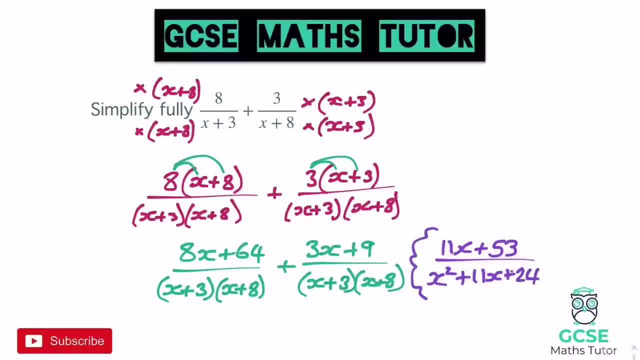 But we'll expand it out and leave that as our final answer there. So we have 11x plus 53.. All over x squared plus 11x plus 24.. Right, there we go. Let's have a look at another one. 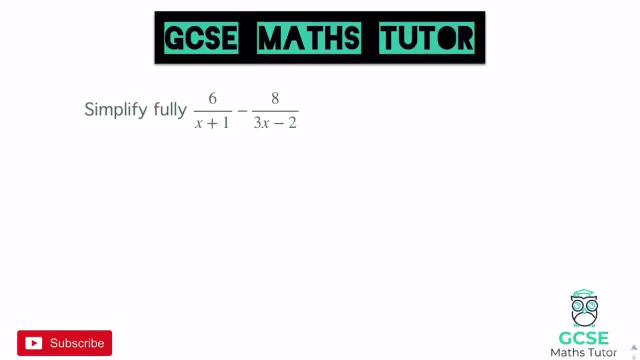 So, moving on to subtraction Now, we're going to take exactly the same approach here, but we are going to be subtracting, So we just need to be careful on one element of this. We're going to have a look at that in a sec. 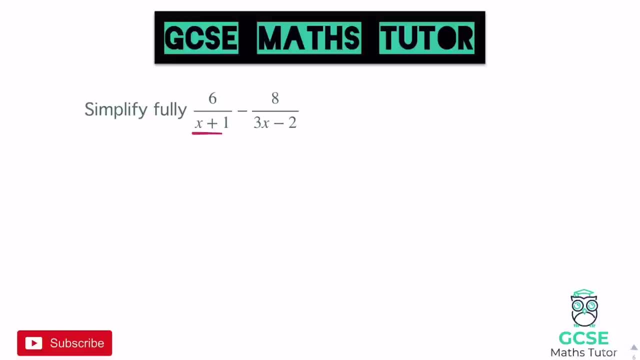 So timesing the right fraction by the left denominator here, timesing it by the x plus 1.. Let's just write that in in fact, as we go. So we're going to times the left as it's on the left. we'll do this one first. 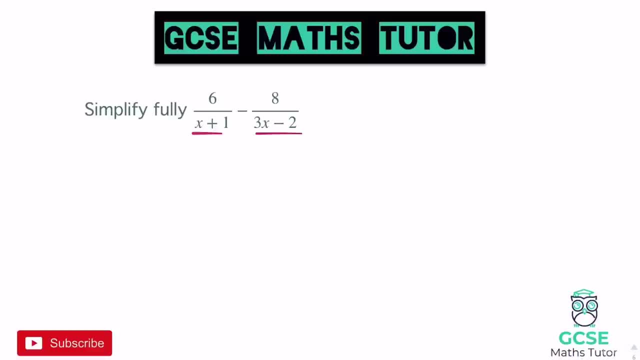 We're going to times the left numerator there by 3x minus 2.. So we'll get 6, lots of 3x minus 2.. All over a double bracket again there. So we'll get x plus 1 and 3x minus 2 on the bottom. 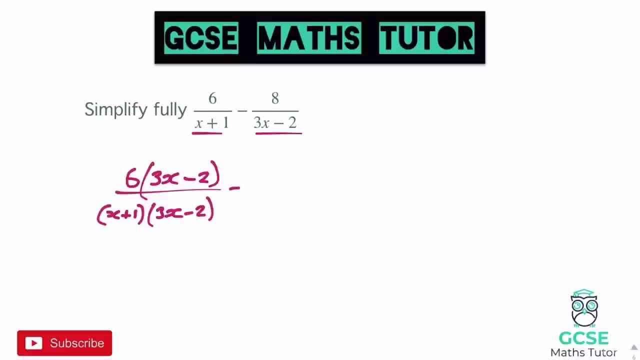 There we go, And we're going to be taking away the next fraction, which is 8. lots of that left denominator x plus 1.. And again all over x plus 1 and 3x minus 2.. There we go. 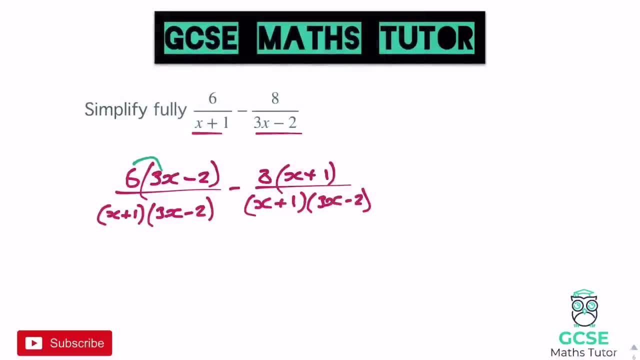 Right. so if we expand this, tidy up the top. So 6 times 3x gives us 18x. 6 times negative 2 gives us negative 12.. There we go, So 18x minus 12. And you know what? 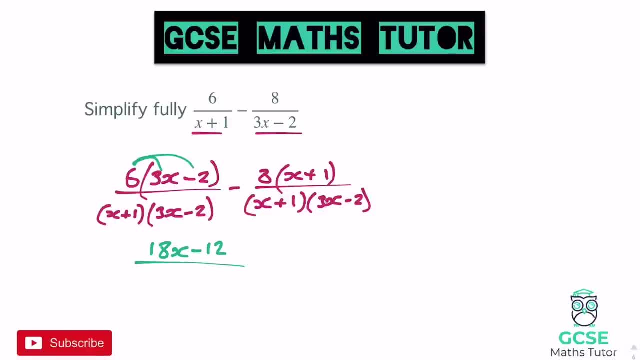 Let's just go and expand the bottom, even though we don't have to. So 3x times x is 3x squared, We're going to get minus 2x, plus 3x, which is going to be plus 1x. 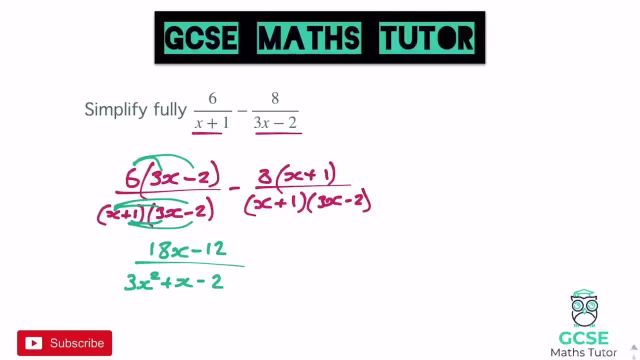 And then 1 times minus 2 is minus 2.. Right, there we go And we're going to be taking away. expanding the top here gets us 8x and plus 8.. And again, that's all over that quadratic there. 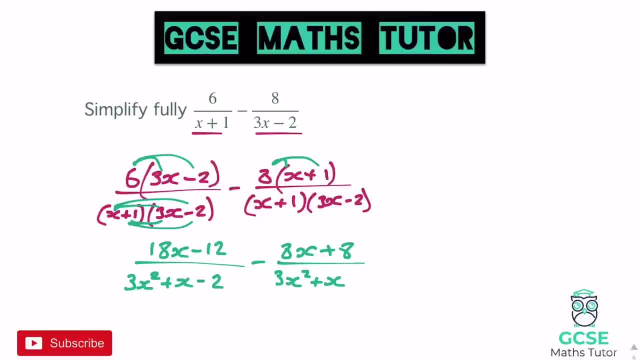 3x squared plus 1x minus 2.. Right, so we just need to finish this off, We just need to tidy up the tops And we need to just be very, very careful when it's a takeaway here. So we've got 18x and we're taking away the 8x. 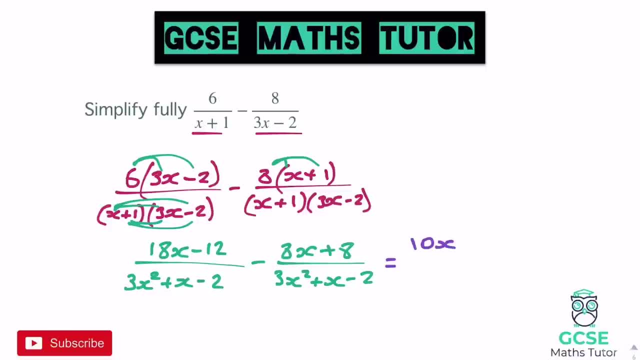 So 18x take away 8x leaves us with 10x, And you've got to be careful as well, because we are taking away this fraction here. We can always again imagine this is in brackets and we're going to be taking away both of these pieces. 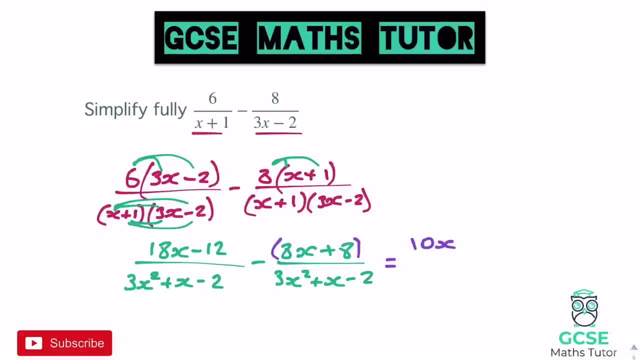 So we've already taken away the 8x, but now we've got negative 12, and we're taking away positive 8.. So negative 12, take away the 8.. Being careful not to add the 8 there. We are taking away both those pieces on the numerator. 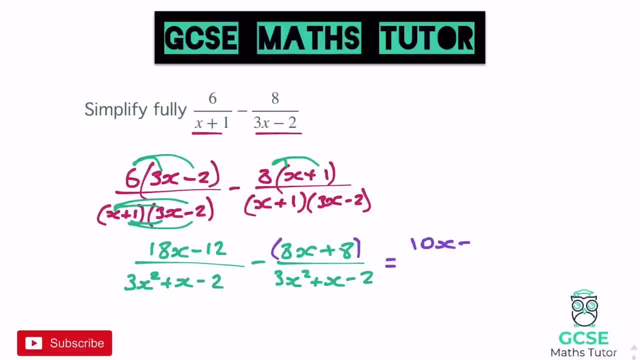 So negative 12, take away 8, gives us negative 20.. So 10x minus 20.. There we go, And on the bottom we've got our quadratic there: 3x squared plus x minus 2. And there is our final answer. 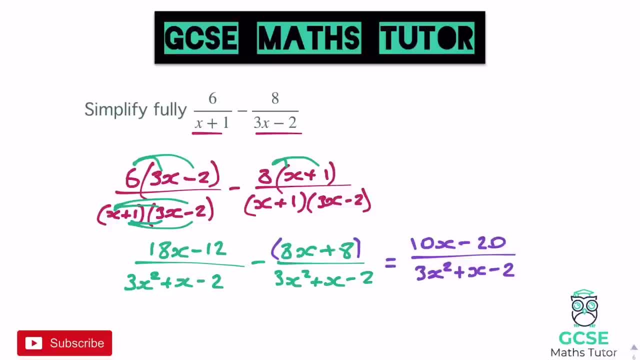 OK, finishing that off. So again, you can leave the bottom factorised. Sometimes it is going to require you to expand it out. I tend to just expand it out anyway. It doesn't take too much time to expand that out and I just prefer writing it. 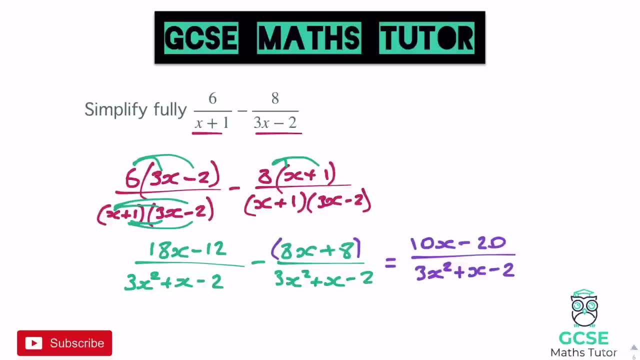 You know, in all these steps, once it's been expanded, rather than writing out all the brackets, there's a little bit less to write. OK, so right, here's something for you to have a go at. OK, so there's two questions there. 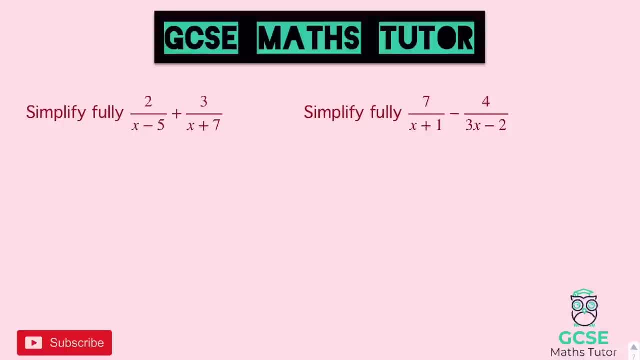 Have a go. Do just be very careful of the takeaway on that right question there. But pause the video. have a go and we'll go over the answers in a sec. OK, so the first one. We have 2 lots of x plus 7 on the top. 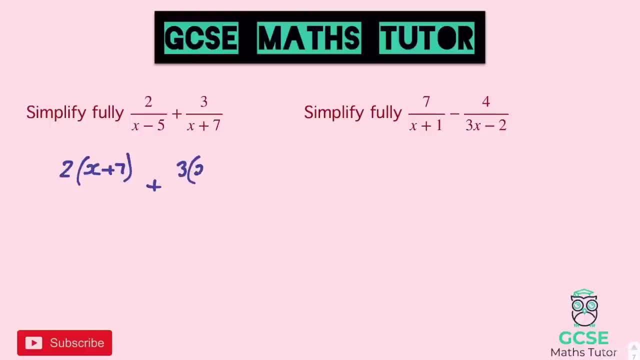 Adding this whole fraction to 3, lots of x minus 5.. There we go On the bottom. I'm just going to expand that out straight away. We're going to get x squared. plus 7x minus 5x is plus 2x minus 35.. 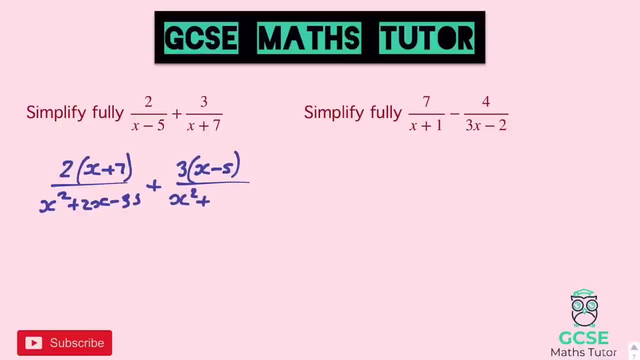 5 times 7, there we go, And the same on the other one: x squared plus 2x minus 35.. If we tidy up the tops, let's have a look. Just to save a bit of time here, I'm just going to expand it all out here. 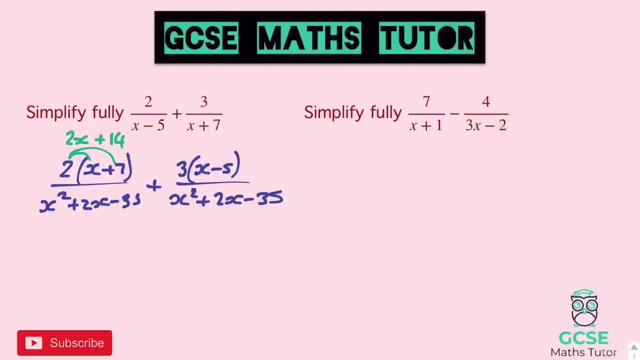 So we get 2x plus 14 on the top, And here we get 3x minus 15.. There we go. So if we write this all out, we've got 2x. add to 3x, which gives us 5x. 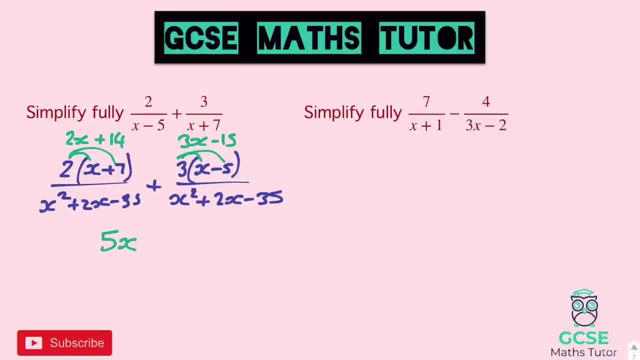 And we've got the 14, add the negative 15.. And 14 add negative 15 is 14. take away 15, which gives us minus 1.. And that's all over that quadratic there, x squared plus 2x minus 35.. 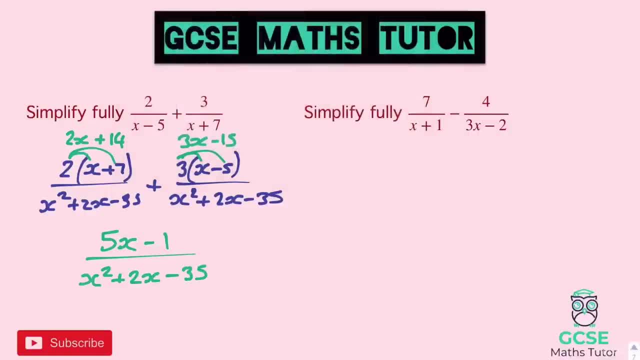 There we go. there's our first one. On to the next one. We have 7 lots of 3x minus 2.. And we are going to be taking away 4 lots of x plus 1 all over the quadratic there. 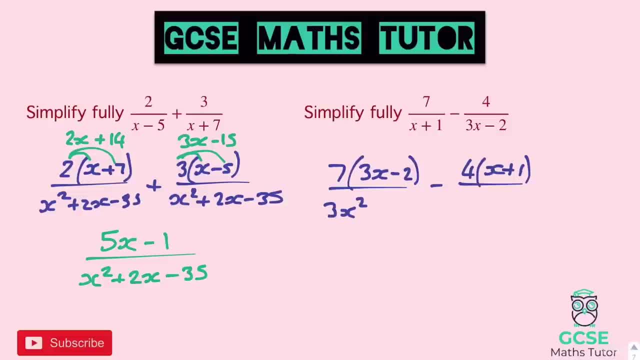 which is 3x squared. Let's have a think Minus 2x plus 3x, which gives us plus x minus 2.. There we go, So 3x squared plus x, minus 2.. Right, expanding those out. 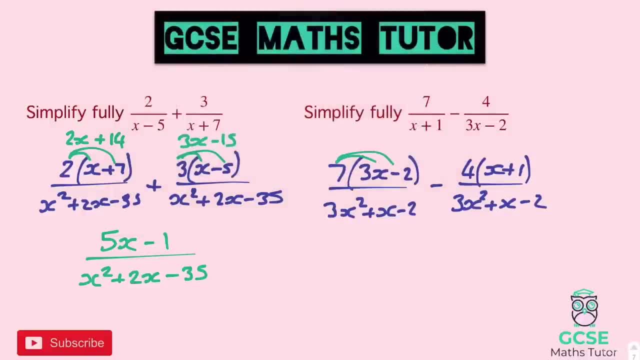 We get 21x minus 14 there, So 21x minus 14.. And here we get 4x plus 4.. OK, So tidying this up, don't forget: it's a take away, So 21x. take away the 4x gives us 17x. 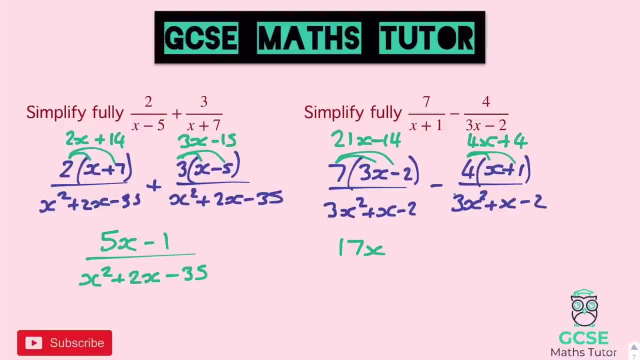 And we've got negative 14. take away the 4,, which leaves us with negative 18.. Negative 14: take away the positive 4. Leaves us with negative 18. And that is all over 3x squared plus 1x minus 2.. 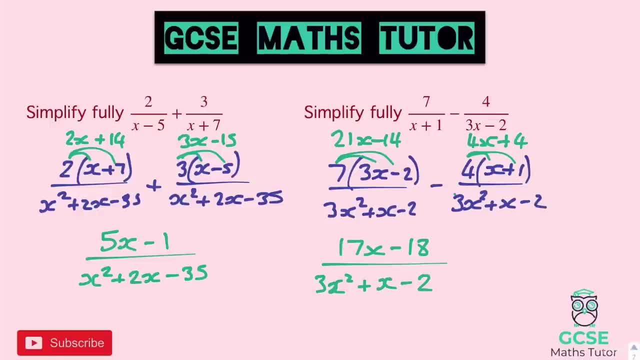 There we go and there's our final answer. Right? so one more last little thing we're going to have a look at. We're going to have a look at dividing with an algebraic fraction quickly. OK, so this question here. we've got quite a lot going on. 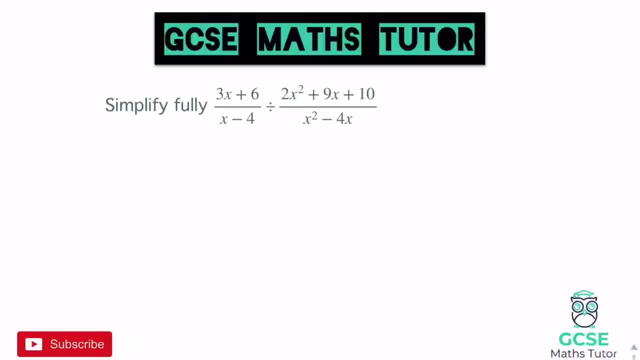 We've got one fraction divided by another and it says: simplify it fully. Now, if we have a look at what we've got to do, we know when we're dividing fractions we have to keep the first one and times it by the reciprocal. 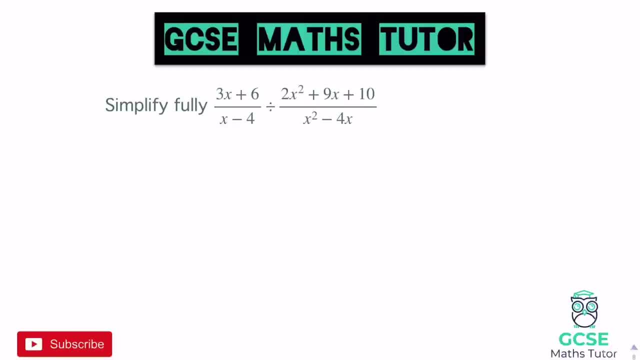 So flipping the second one over, So we can just write that out straight away if we want. I'm just going to factorise any in the process, though, so I'm just going to do that here before we actually write anything down. So that factorises by 3, and that would leave you with x plus 2.. 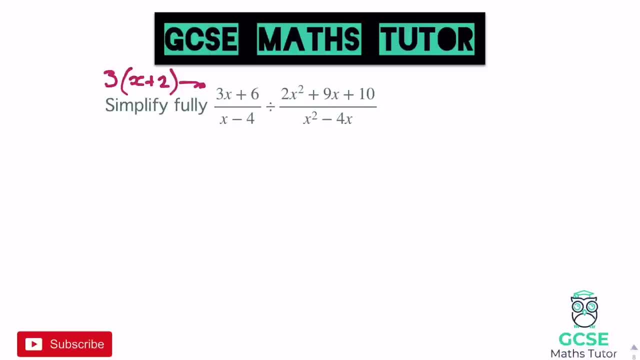 The bottom there doesn't factorise, so that will stay as it is. So we can write this out now. So we've got 3 lots of x plus 2, all over x minus 4. And we're going to times that by the flipped version. 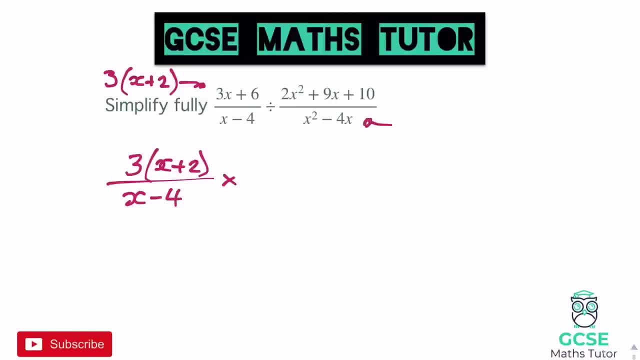 but let's see if we can factorise them first. So the bottom here is quite a nice one: Factorises by x And we get x minus 4.. So that's going to now be on the top when we flip it over. 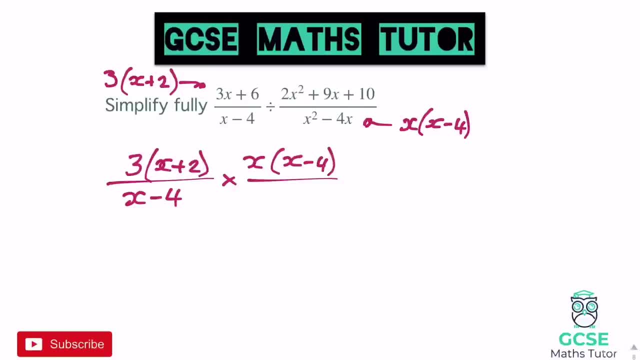 So we have x brackets, x minus 4.. And this one here we're going to have to factorise this as well. So we've got 1 and 10, or 2 and 5.. Let's have a look Now. one of them is going to be a 2x, because it's 2x squared. 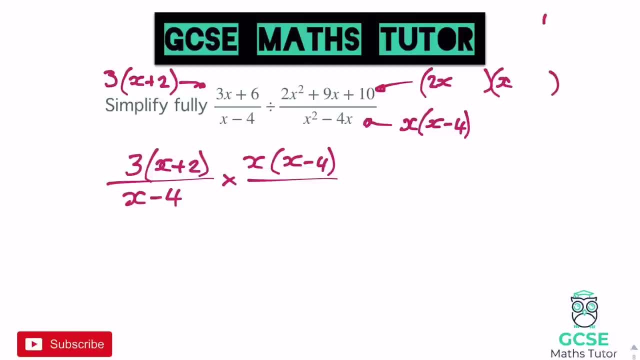 And one's an x Right. so let's write these down. We've got 1 and 10, or 2 and 5. And we're trying to make 9.. So let's have a think We could double the 2.. 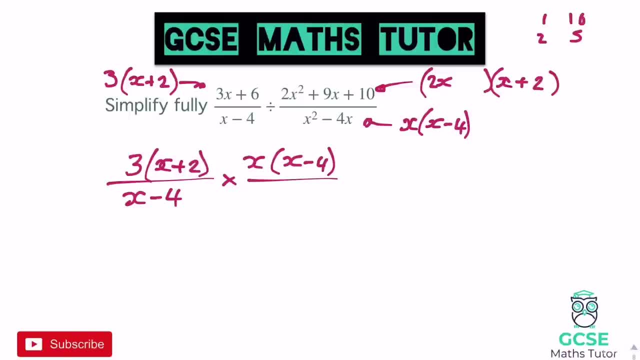 There we are. That works. So double the 2.. So 2 in the other bracket Plus 2. That would make 4.. And plus 5 over here, And 4 plus 5 would make 9.. So we can put that on the bottom now. 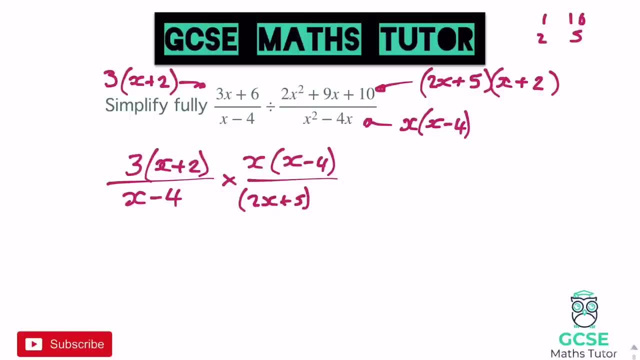 So we've got 2x plus 5. And x plus 2.. There we go. Now, if you think about what we'd have to do here with times in fractions, if we times fractions we just times the top, times the bottom. 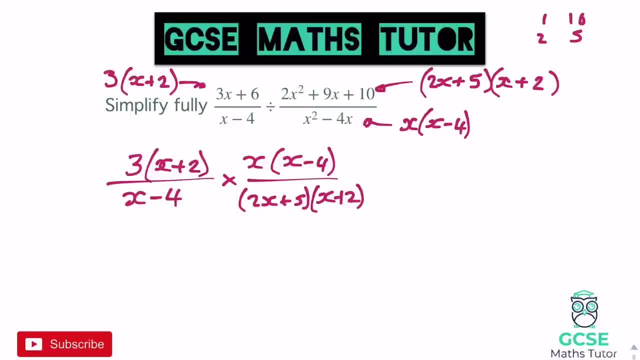 So essentially, everything there on the top is going to be on the top of our fraction And everything on the bottoms of those two fractions are going to be everything on the bottom. So what we can do at this point, we can actually cross cancel some of these. 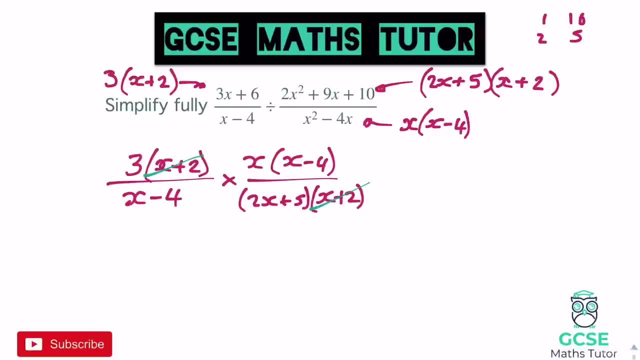 And if you have a look, we've got an x plus 2 there and an x plus 2 here, Because obviously, if we actually did multiply these together, one would be on the top, one would be on the bottom. So we can cross cancel them before doing so. 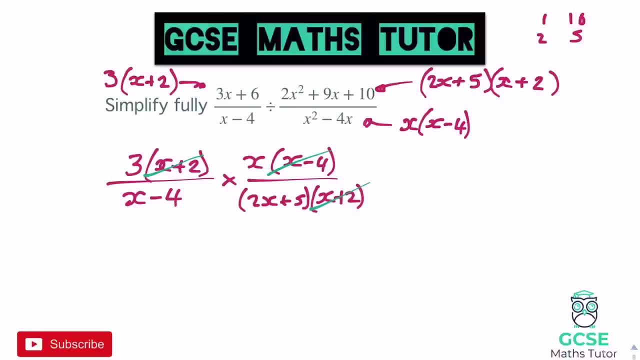 So they're gone. We can also cancel this x minus 4. So that's gone as well. Obviously, on the bottom there, that's the only thing there, So that would turn into a 1. And everything else has something with it. 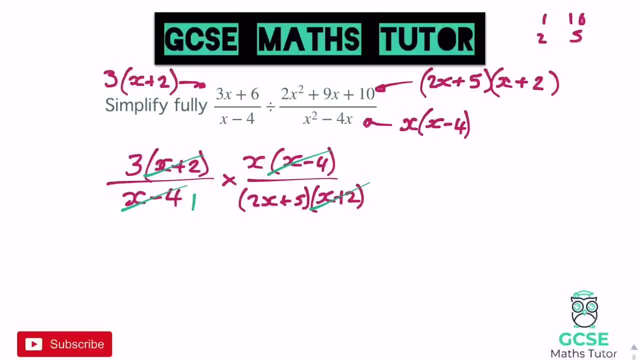 So if we times together what we've got on the top now, we've got a 3 and an x on the top of those two fractions. So 3 times x is 3x, And on the bottom there we've got 1 multiplied by 2x plus 5.. 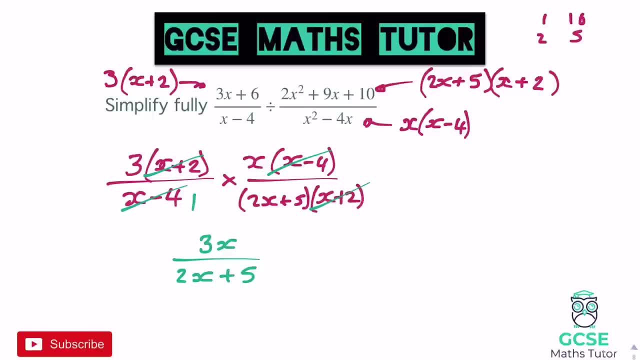 So that's just 2x plus 5.. There we go. So that simplifies all the way down to that. Okay, so obviously, just have a look When you're doing one of these dividing fractions or any of these algebraic fractions. 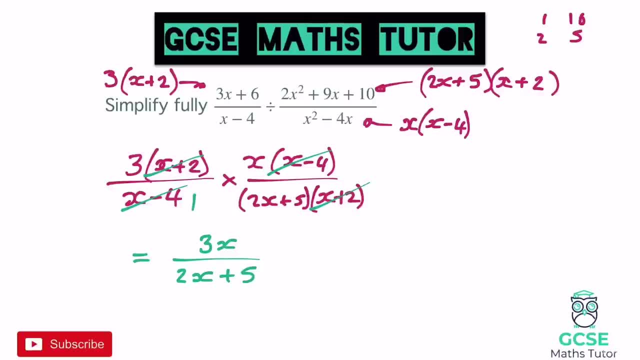 look to factorise anything you can And just follow normal fraction rules. So here we factorised everything and then times it by the reciprocal, flipping it over and just cross, cancelled any common brackets there before multiplying them together, just to say. 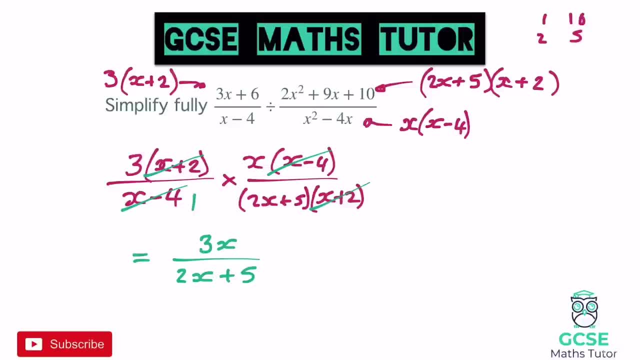 we're just going to write it out and then cancel them off. Right, here's one for you to have a go at. Okay, so have a go at this question. Pause the video there. We'll go over the answer in a sec. 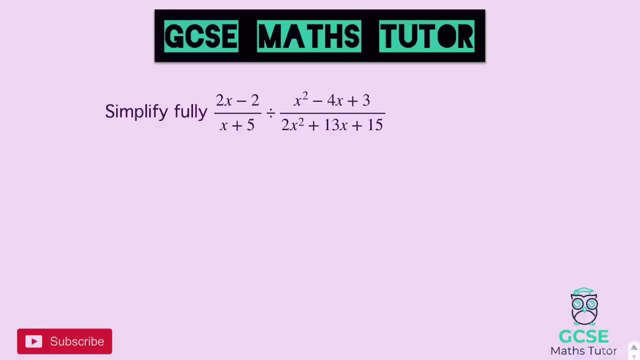 Right, okay. so let's have a look. The top of that, left one, factorises by 2.. So if we factorise that by 2, we get two lots of x minus 1. And on the bottom, that doesn't factorise. 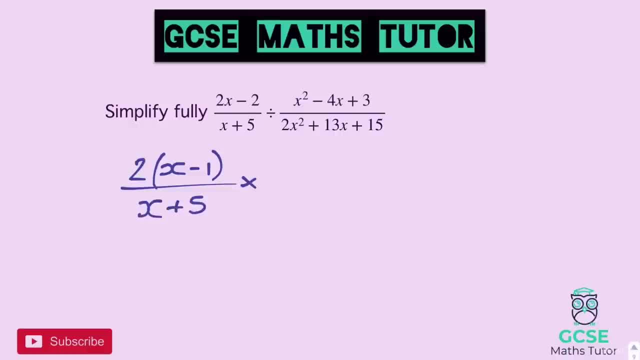 just x plus 5.. And we're going to times that by this one flipped over. so let's factorise this. So what's that? for make 3? x minus 3 and x minus 1.. There you go, x minus 1.. 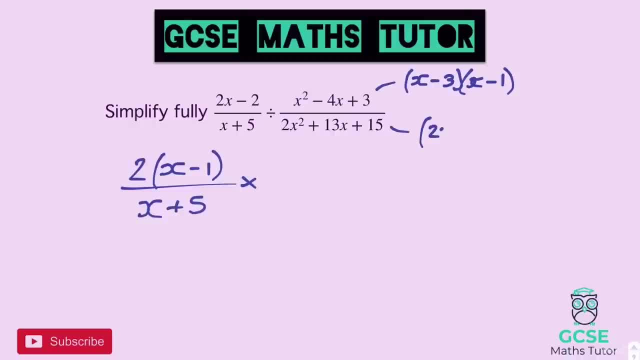 And on the bottom there let's see how that factorises. So 2x squared, so we've got a 2x and an x Numbers. that times to make 15, we've got 1 and 15, or 3 and 5.. 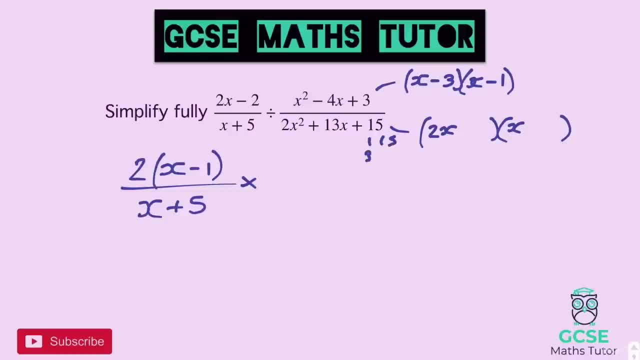 Trying to make 13,. so we want to double the 5 and add the 3.. So double the 5, put that over there, And then a 3 on its own, And there's that. So let's flip them over. 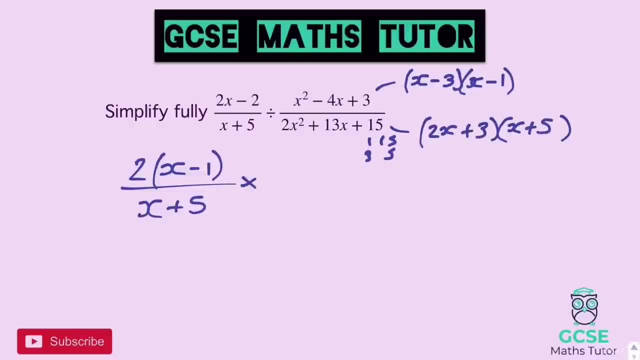 We have 2x plus 3, and x plus 5.. And on the bottom there we have x minus 1, and x plus 5.. And on the bottom there we have x minus 1, and x plus 5.. 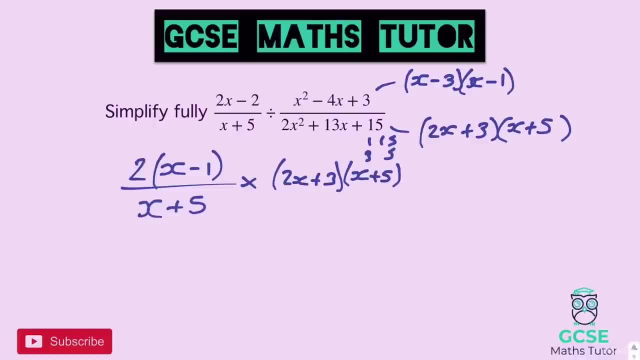 And on the bottom there, we have x minus 1, and x plus 5.. And on the bottom there, we have x minus 3, and x minus 1.. There we go Right. so, thinking about this, let's see what we can cancel off. 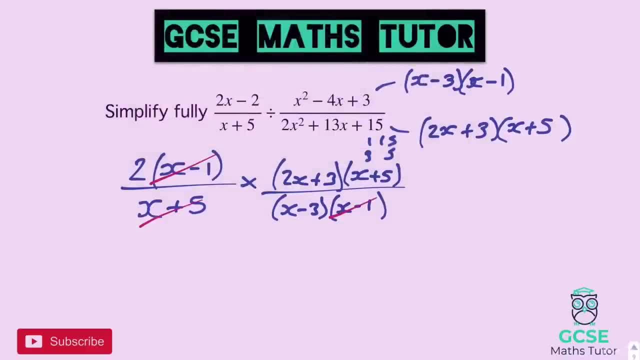 We've got the x minus 1 and the x minus 1.. And we've got the x plus 5 and the x plus 5.. Obviously, that becoming 1 now. So we've got 2. lots of what's on the top there. 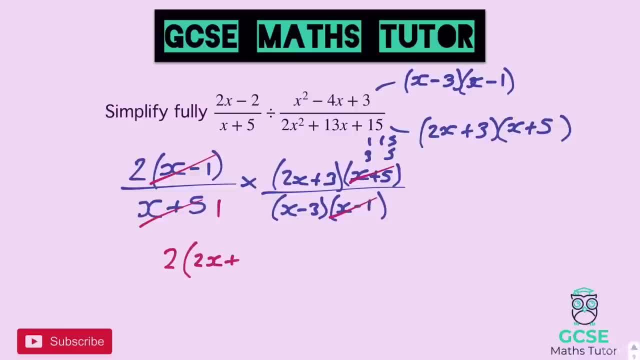 2, lots of 2x plus 3, just multiplying the tops, multiplying the bottoms, And on the bottom we have 1 lot of x minus 3, which we can just write as x minus 3.. There we go. 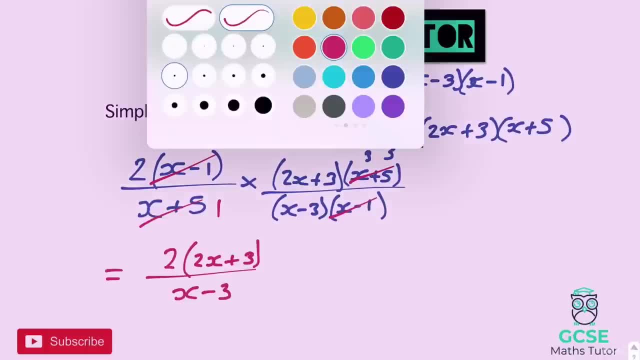 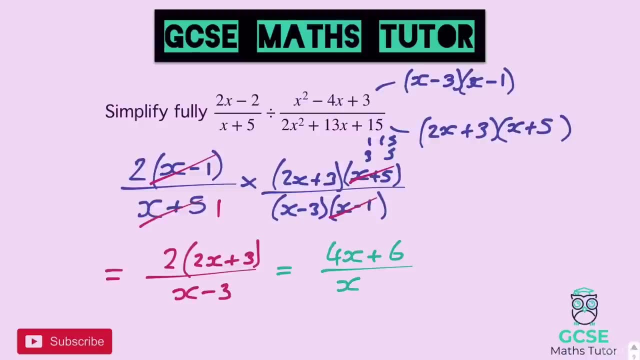 That would be fine to leave our answer like that, but we could actually expand it as well. So if we expand the top, we would have 4x plus 6 over x minus 3.. Okay, And that's absolutely fine for us to just leave it like that. 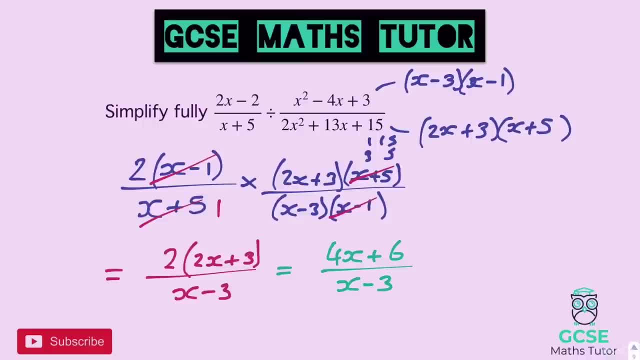 Or we could have left it factorised as well. but both answers there would be absolutely fine. But there we go. A little selection of different algebraic fractions: there We did simplifying with all the kinds of different examples. there We did a little bit of adding. 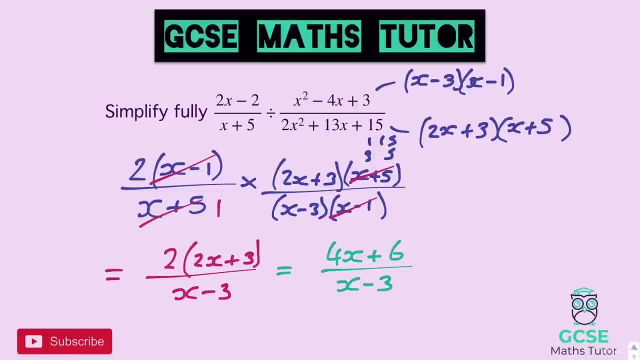 and subtracting, obviously with some unique examples. There we go. So there's quite a lot of different examples there, but the principle stays the same, no matter what, And a little bit of dividing there. Obviously, if you are multiplying, we did some multiplying as well. 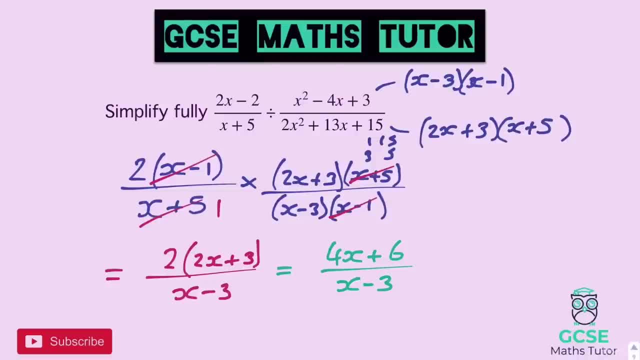 in that second step. even though we were dividing, Same principles would apply for multiplying them. But there we go. There's a little bit of a selection of different algebraic fractions, But if you found that useful, if it was helpful, please like.